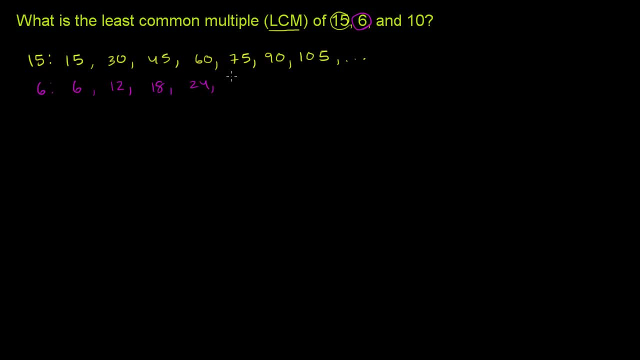 3 times 6 is 18.. 4 times 6 is 24.. 5 times 6 is 30.. 6 times 6 is 36.. 7 times 6 is 42.. 8 times 6 is 48.. 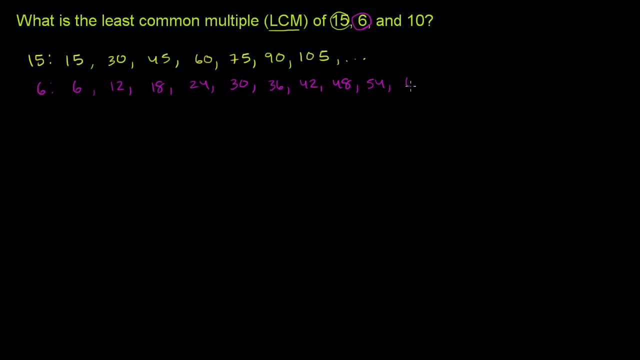 9 times 6 is 54.. 10 times 6 is 60.. 60 already looks interesting because it is a common multiple of both 15 and 60. Although we have two of them over here: We have a 30 and we have a 30.. 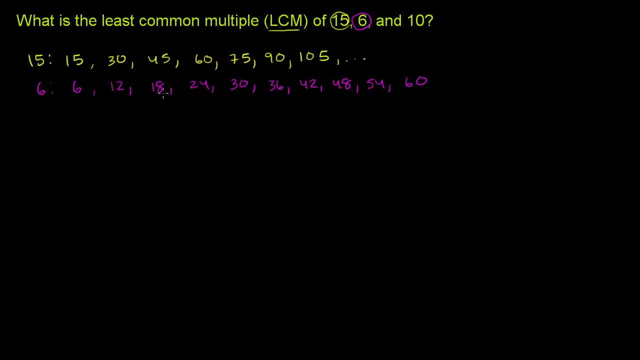 We have a 60 and a 60. So the smallest common multiple. So if we only cared about the least common multiple of 15 and 6, we would say it's 30. So let me write this down as a kind of intermediate. 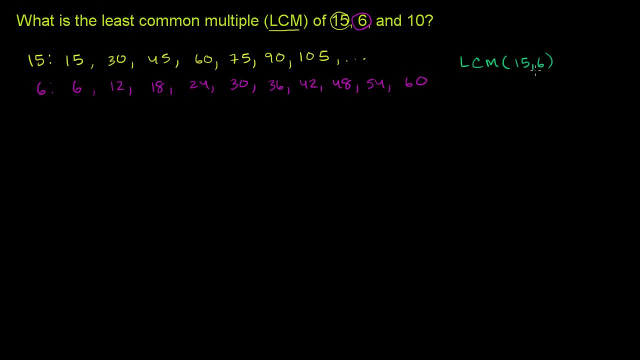 The LCM of 15 and 6, so the least common multiple, The smallest multiple that they have in common we see over here, 15 times 2 is 30. And 6 times 5 is 30. So this is definitely a common multiple. 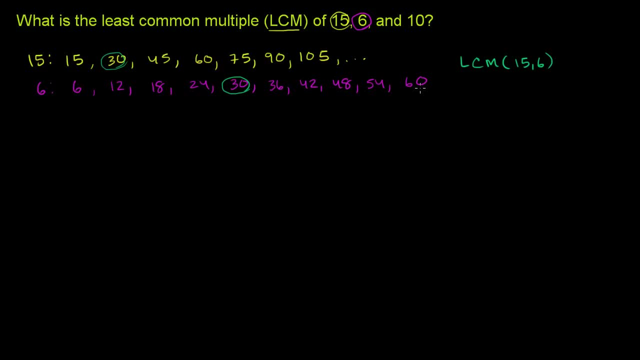 And it's the smallest of all of their common multiples. 60 is also a common multiple, but it's a bigger one. This is the least common multiple, So this is 30.. We haven't thought about the 10 yet, So let's bring the 10 in there. 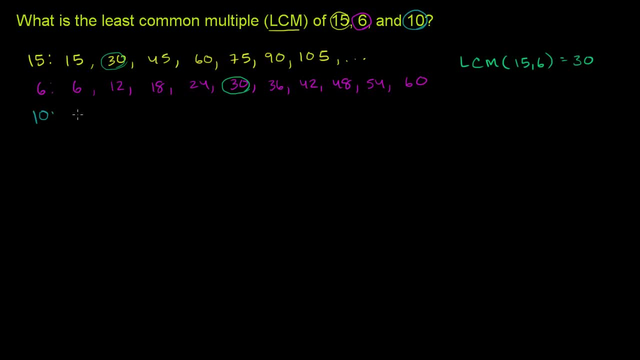 And I think you already see where this is going. Let's do the multiples of 10.. There are 10, 20, 30. 40.. Well, we already went far enough, because we already got to 30. And 30 is a common multiple of 15 and 6.. 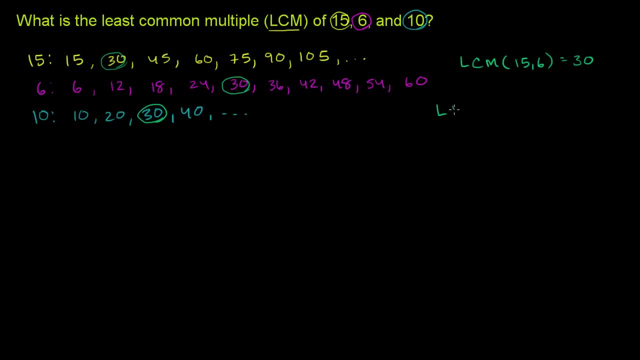 And it's the smallest common multiple of all of them. So it's actually the fact that the LCM of 15,, 6, and 10 is equal to 30. Now this is one way to find the least common multiple. 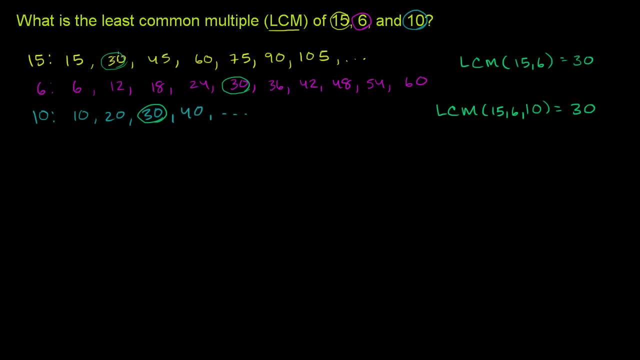 Literally just look at the multiples of each of the number and then see what the smallest multiple they have is in common. Again, another way to do that is to look at the prime factorization of each of these numbers, And the least common multiple is the number. 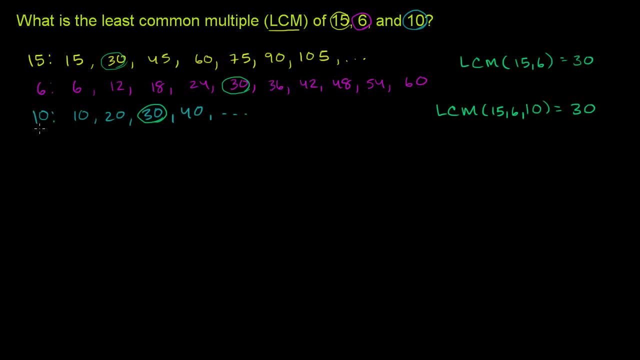 that has all of the elements of the prime factorizations of these and nothing else. So let me show you what I mean by that. So you could do it this way. Or you could say: 15 is the same thing as 3 times 5.. 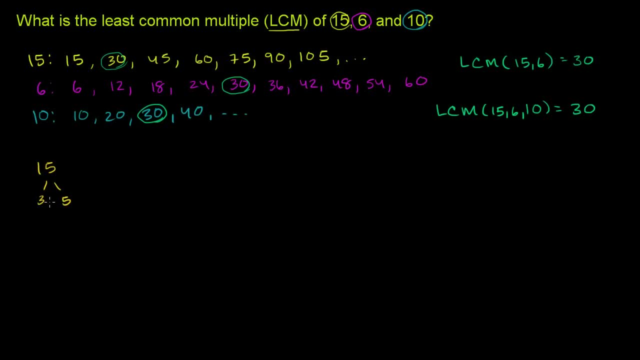 And that's it. That's its prime. factorization: 15 is 3 times 5.. Both 3 and 5 are prime. We can say that 6 is the same thing as 2 times 3.. That's it. 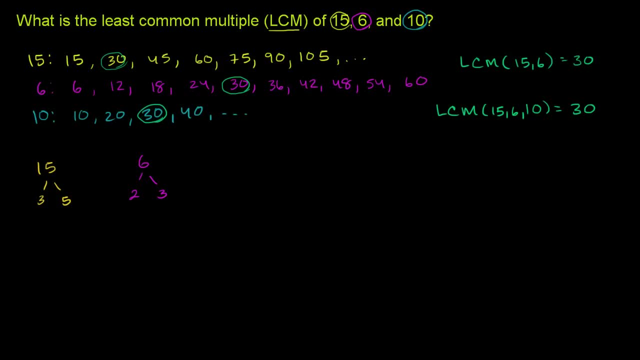 That's its prime factorization. Both 2 and 3 are prime. And then we can say that 10 is the same thing as 2 times 5.. That's it: Both 2 and 5 are prime. So we're done factoring it. 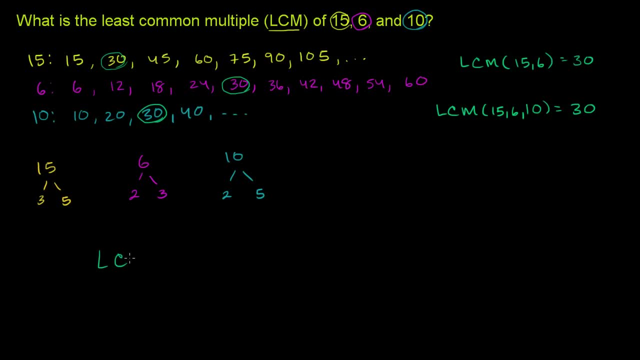 And so the least common multiple of 15,, 6, and 10 just needs to have all of these prime factors, And what I mean to be clear is, in order to be divisible by 15,, it has to have at least one prime factorization. 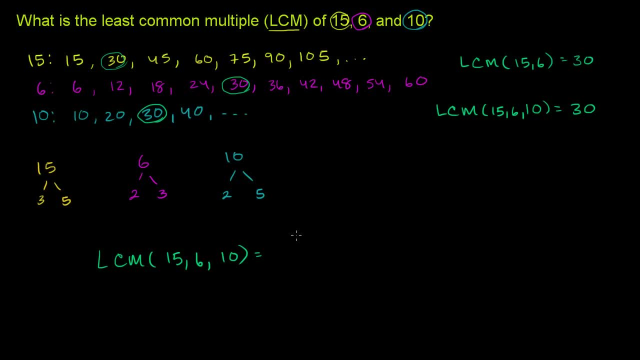 So it has to have at least one 3 and one 5 in its prime factorization. So it has to have at least one 3 and at least one 5.. By having a 3 times 5 in its prime factorization. 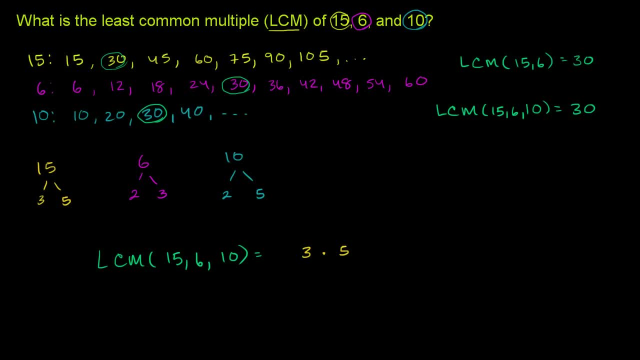 that ensures that this number is divisible by 15.. To be divisible by 6,, it has to have at least one 2 and one 3.. So it has to have at least one 2.. And we already have a 3 over here. so that's all we want. 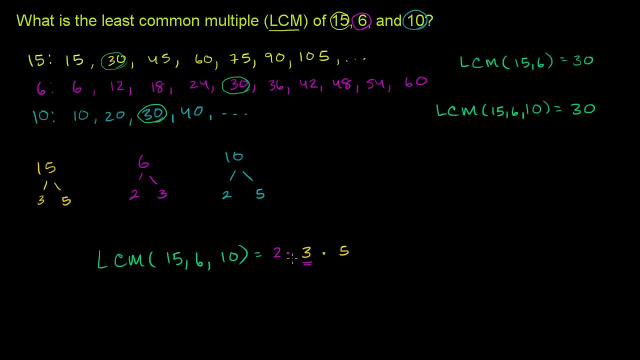 We just need one 3.. So one 2 and one 3, this 2 times 3, ensures that we are divisible by 6. And let me make it clear This right here is the 15. And then to make sure that we're divisible by 10,. 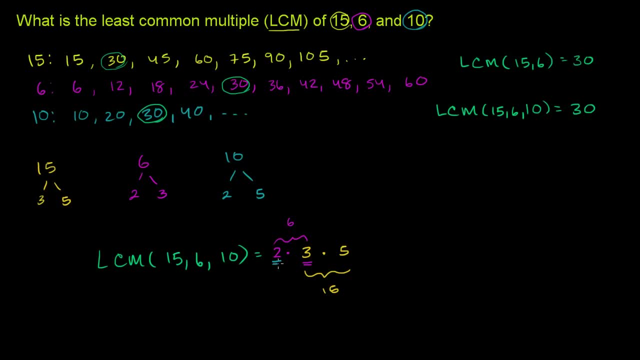 we have to have at least one 2 and one 5.. We have to have at least one 2 and one 5.. These two over here make sure that we are divisible by 10.. And so we have all of them. This 2 times 3 times 5 has all of the prime factors of either 10,, 6, or 15.. 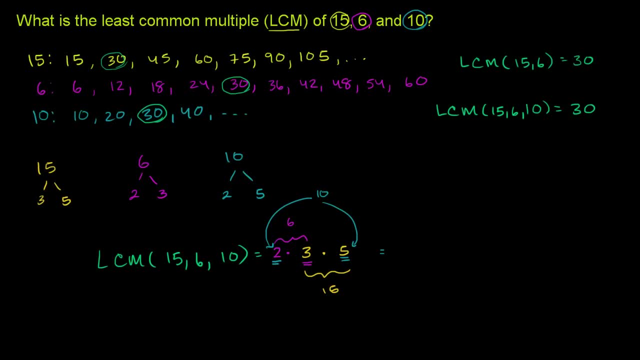 So it is the least common multiple. And so if you multiply this out, you will get 2 times 3 times 5.. 2 times 3 times 5 is the least common multiple, So if you multiply this out, you will get 2 times 3 times 5.. 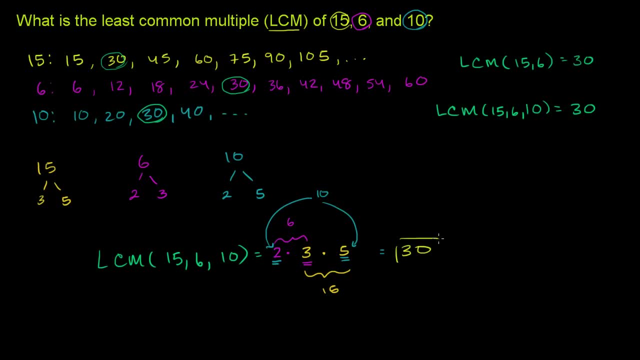 2 times 3 is 6.. 6 times 5 is 30. So either way, hopefully both of these kind of resonate with you and you see why they make sense. This second way is a little bit better, if you're. 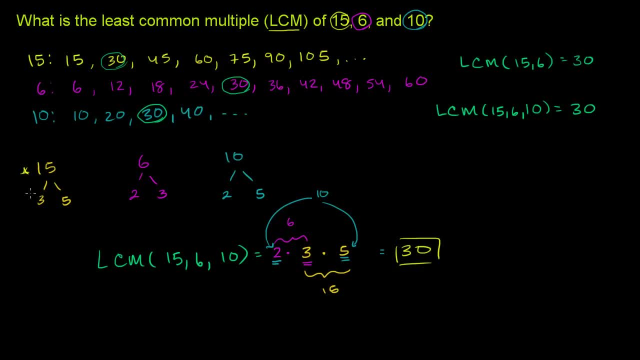 trying to do it for kind of really complex numbers, numbers where you might have to be multiplying it for a long time. Well, either way, both of these are kind of valid ways of finding the least common multiple.